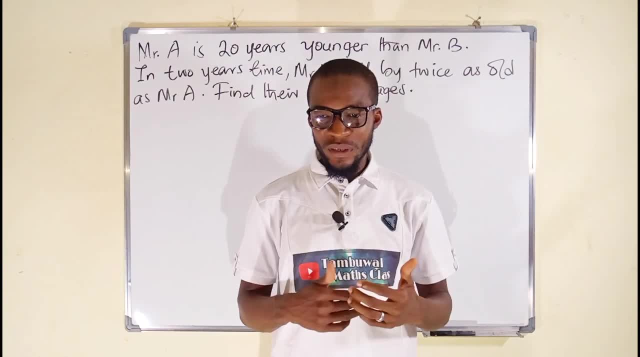 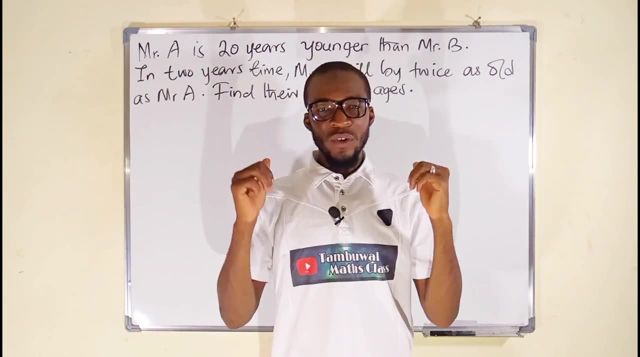 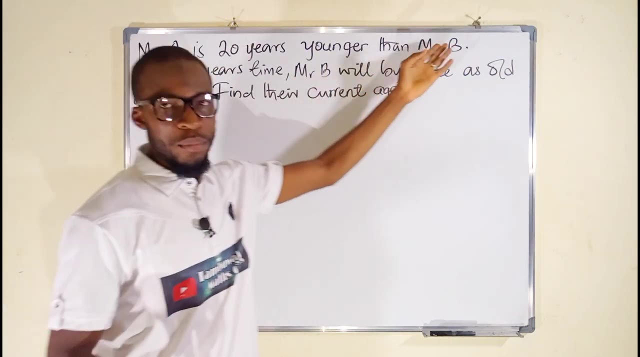 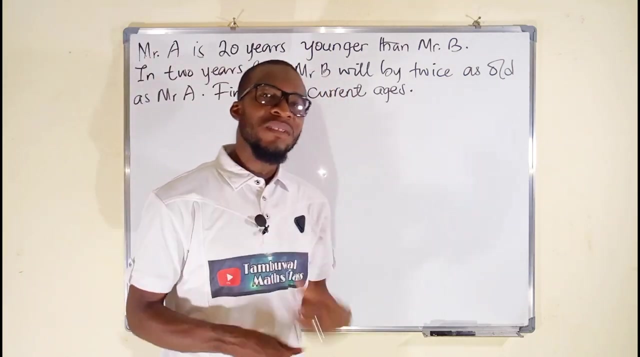 many things. So by next week I think we're going to start with second order linear non-homogeneous differential equations. So back to business. This question reads: Mr A is 20 years younger than Mr B. Take note of that. But in two years coming Mr B will be twice as old as Mr A. 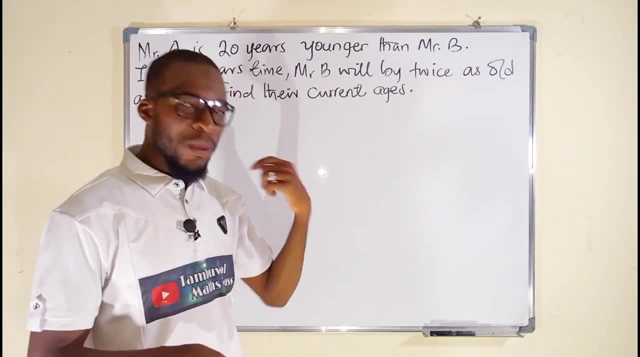 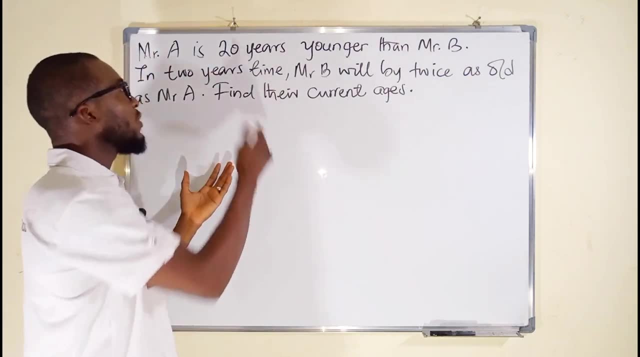 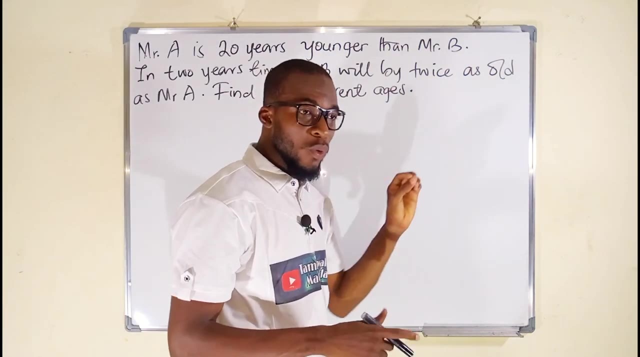 This means that currently Mr B is older than Mr A. Take note of that. We are asked to find their current ages. So currently we don't know their age, But we are asked to find their current edges. but we learned that mr a is 20 years younger than mr b, so it means mr b is older. so 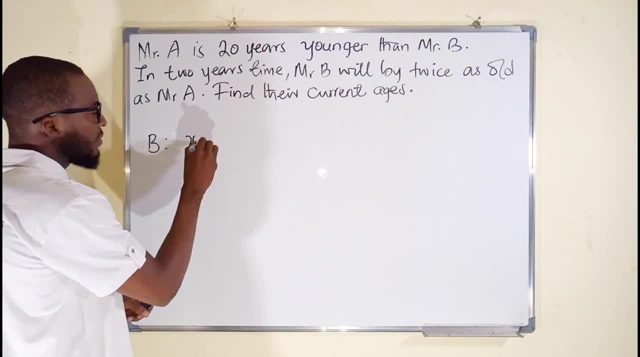 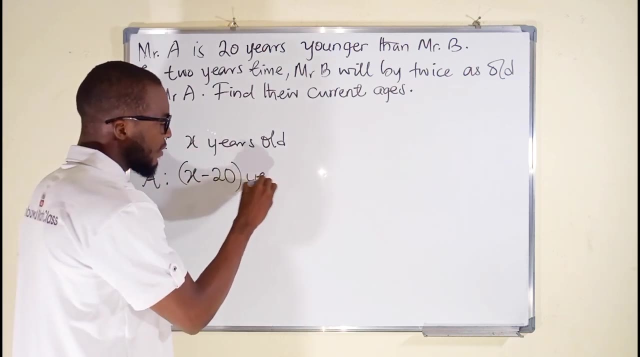 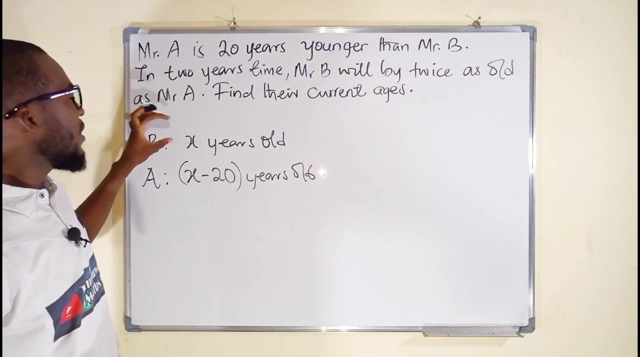 suppose mr b is x, yes, old. what does this mean? it means that mr a will be x minus 20. yes, because we learned that mr b is older. so whatever the age of mr b is, you have to subtract 20 from that to get the age of mr a. let's continue. so this is the current age, or current year. 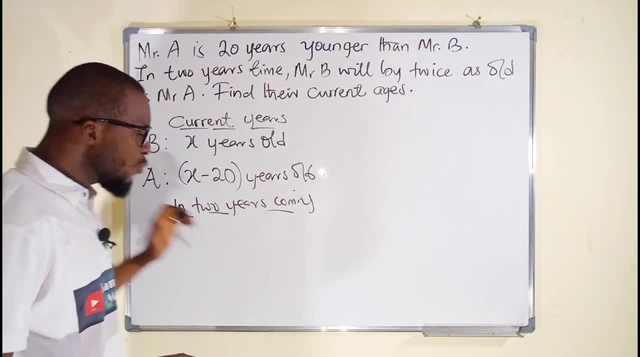 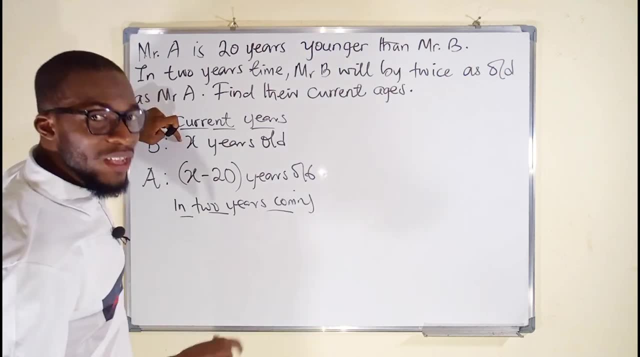 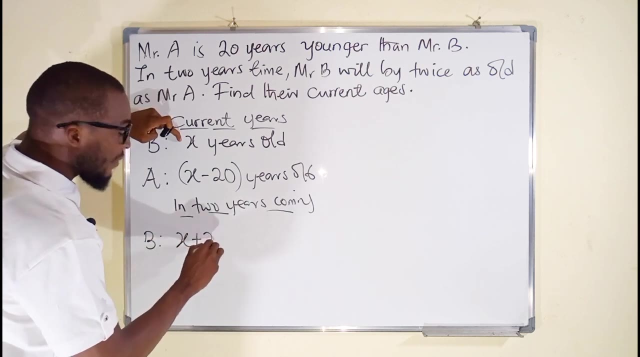 in two years coming. in two years coming, each of them will add two extra. yes, so currently you can see mr b is x years old. therefore, mr b will be x plus two years. after two years, after two years, mr b will be x plus two. that year you can see mr a is x minus 20 old. 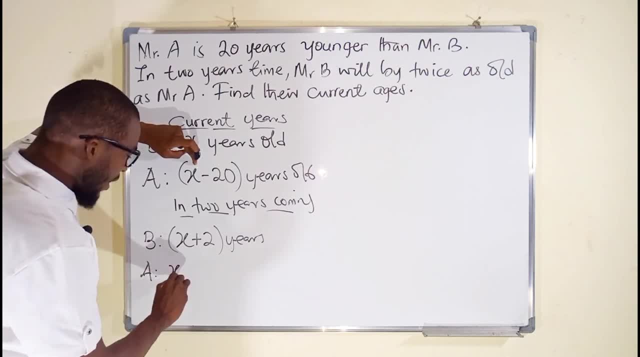 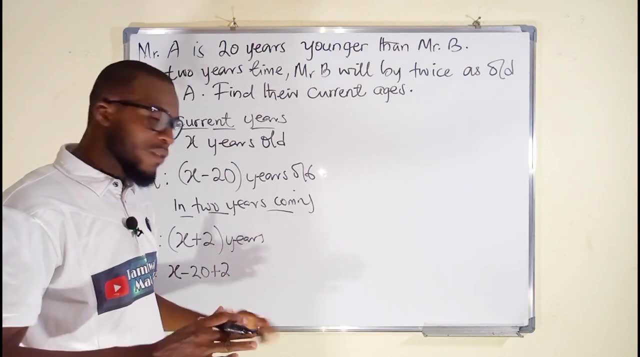 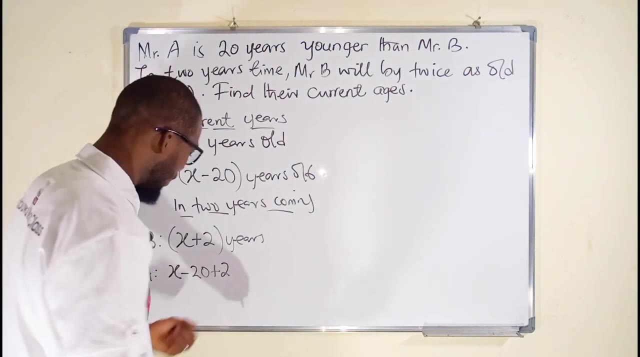 therefore, in two years coming, he will be x minus 20, then also plus, because he is going to add two years extra, which we can simplify. as you can see, we have minus 20 plus 2, which is equal to minus 18.. this is equal to x minus 18.. 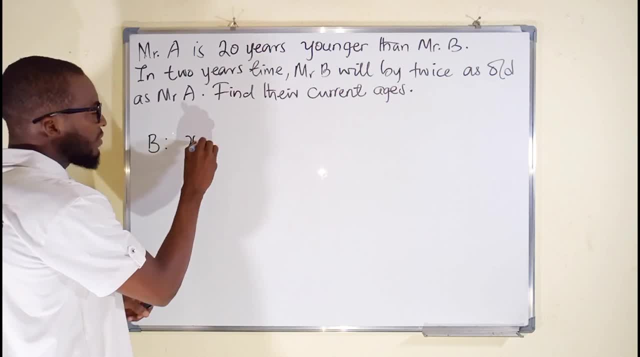 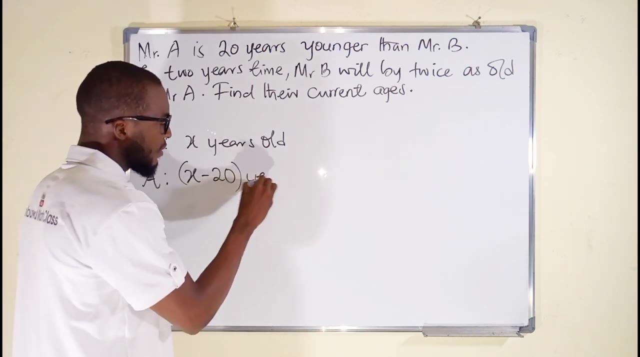 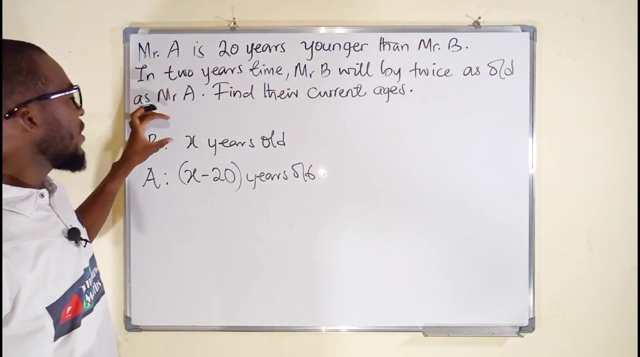 suppose mr b is x, yes, old. what does this mean? it means that mr a will be x minus 20. yes, because we learned that mr b is older. so whatever the age of mr b is, you have to subtract 20 from that to get the age of mr a. let's continue. so this is the current age, or current year. 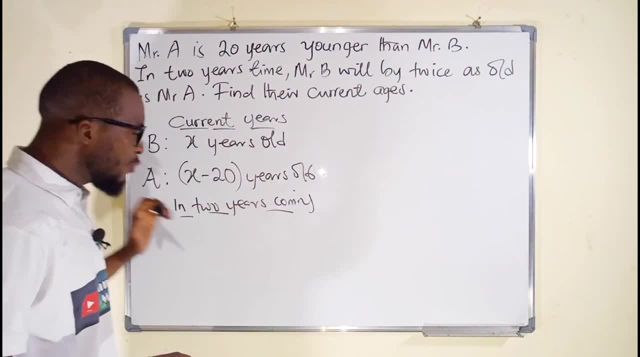 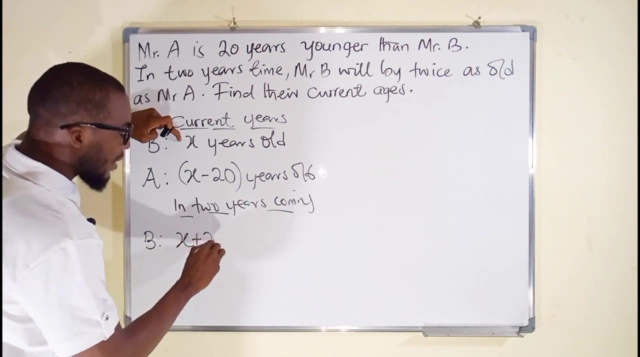 in two years coming. in two years coming, each of them will add two extra. yes, so currently you can see mr b is x years old. therefore, mr b will be x plus two years. after two years, after two years, mr b will be x plus two. that year you can see mr a is x minus 20 old. 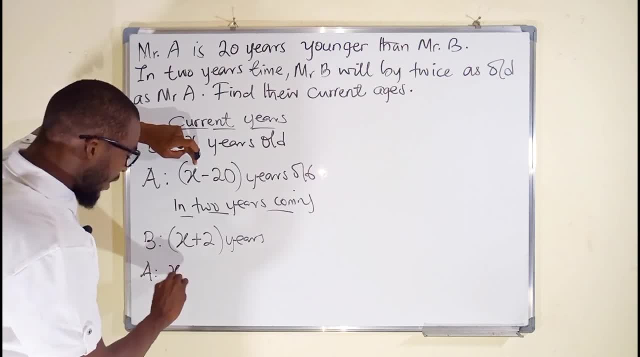 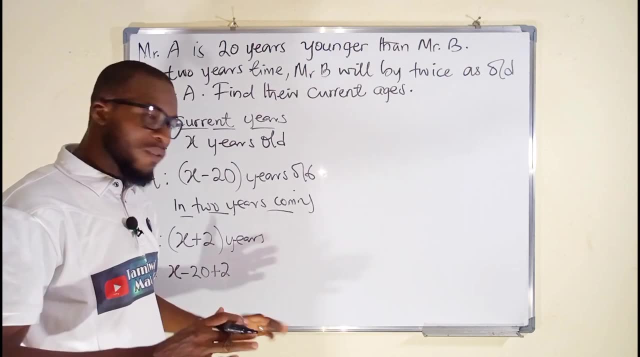 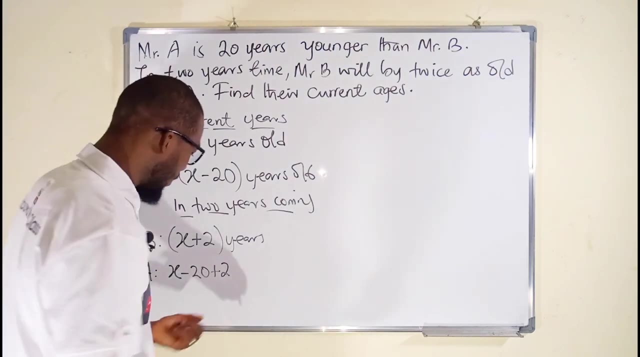 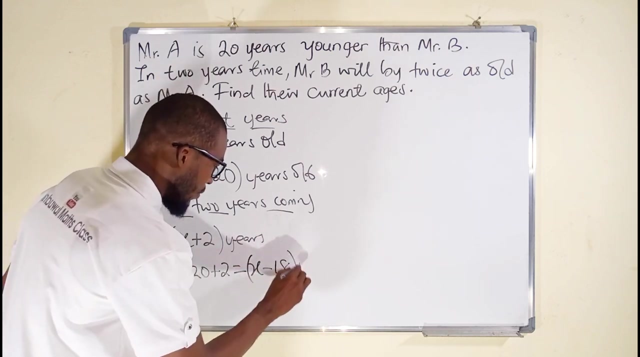 therefore, in two years coming, he will be x minus 20, then also plus 2, because he's going to add two years extra, which we can simplify. as you can see, we have minus 20 plus 2, which is equal to minus 18.. this is equal to x minus 18. yes, 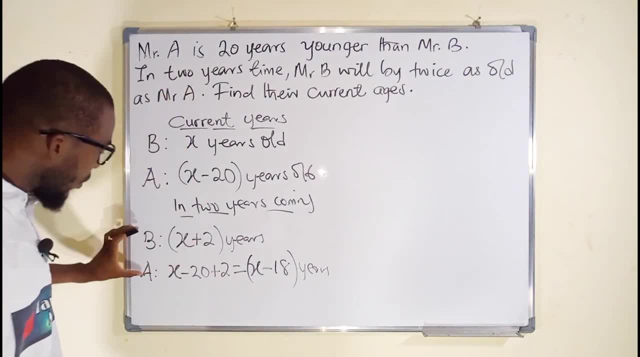 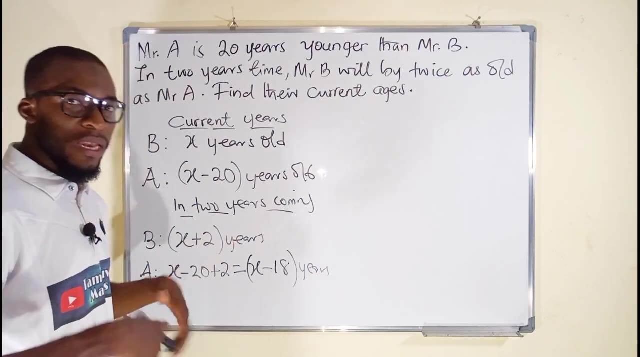 okay, let us continue reading. but we learned that, uh, in the next coming two years, mr b will be twice as old as mr a, So you have to multiply Mr A's age by 2 to get that of Mr B in the next coming 2 years. 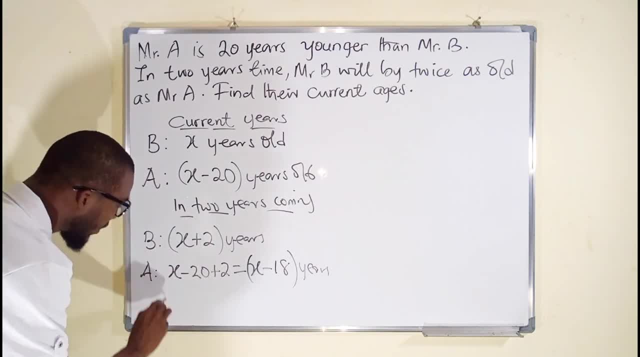 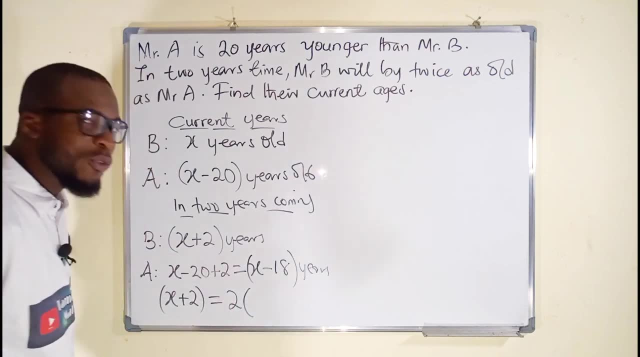 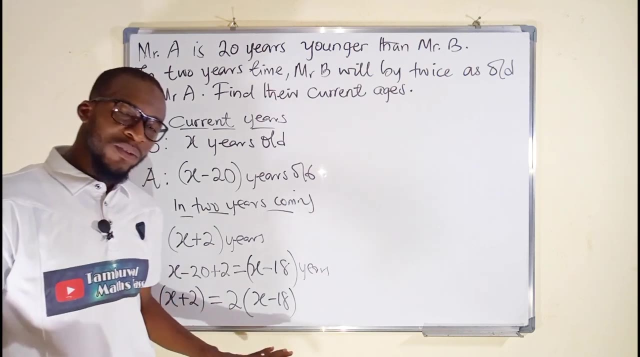 So currently, after 2 years, Mr B, which has this x plus 2 as his age, will be equal to 2 multiplied by the age of Mr A, which we have as x minus 18.. So this is the equation we need to solve for x. 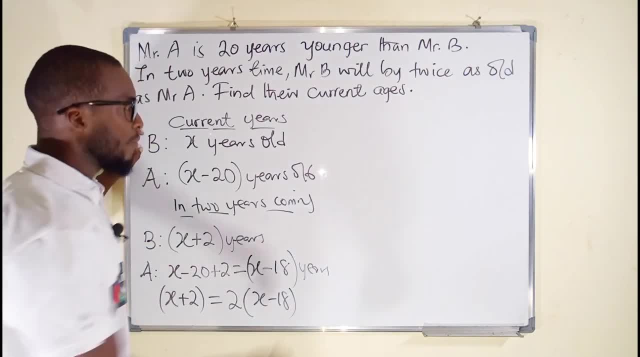 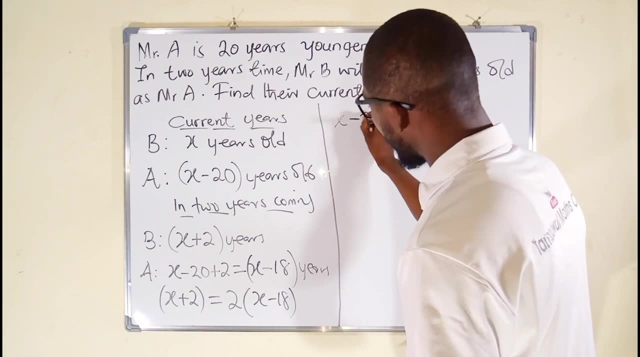 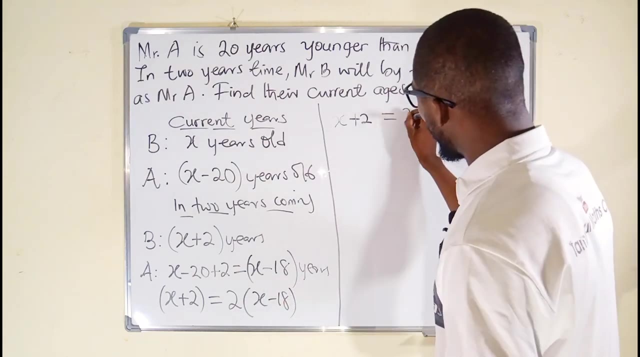 Whatever the value of x is, is said to be the age of Mr B, So let us do it here. You can see we have x plus 2 to the left And to the right we have: 2 multiplied by x is 2x minus 2 multiplied by 18 is 36.. 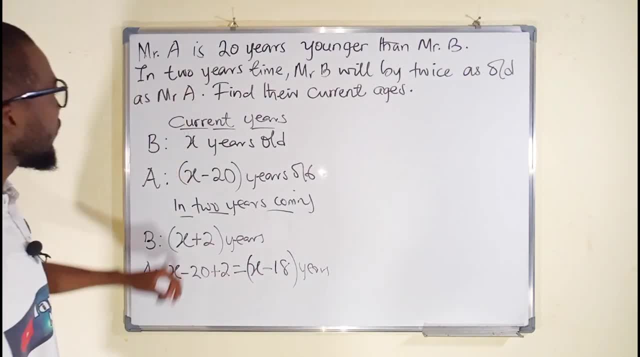 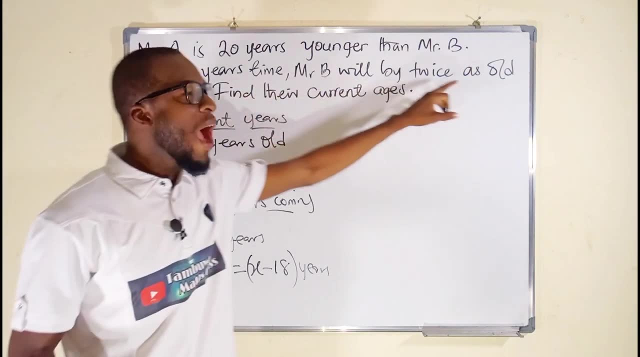 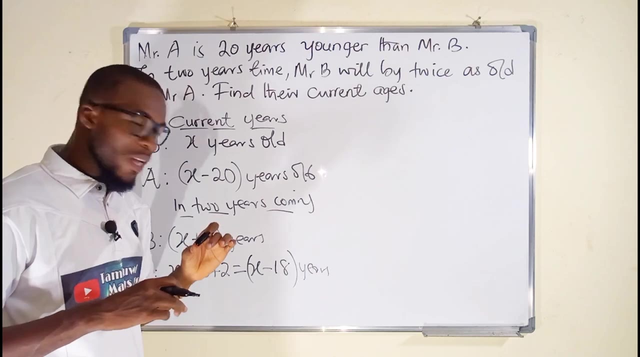 yes, okay, let us continue to read it. but we learned that, uh, in the next coming two years, mr b will be twice as old as mr s. mr a to n is aellow A, So you have to multiply Mr A's age by two to get that of Mr B in the next coming two years. 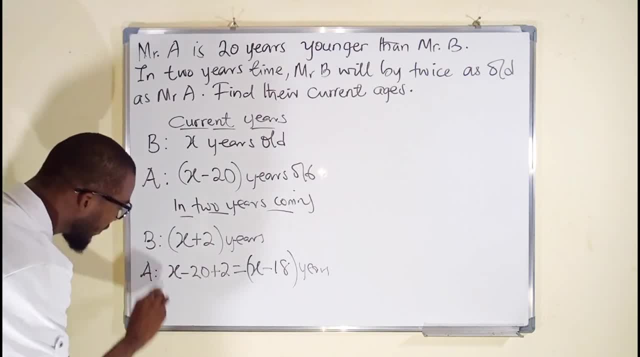 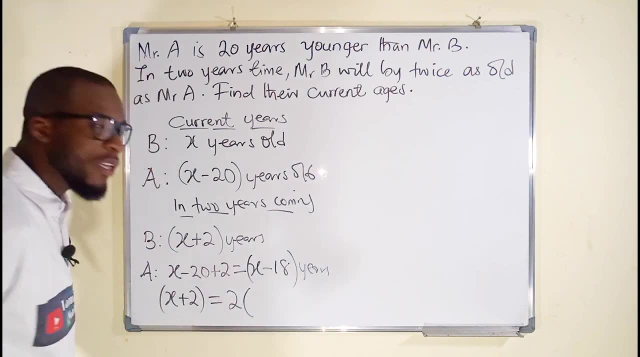 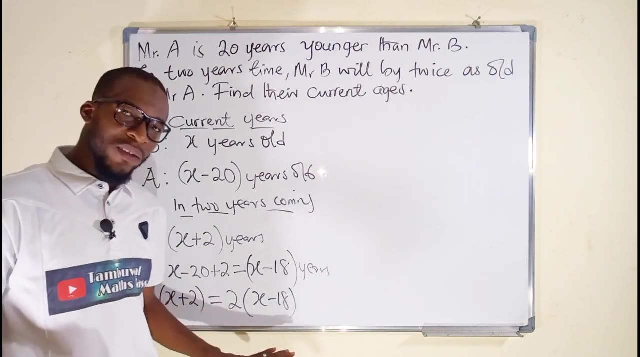 So currently, after two years, Mr B, which has this x plus two as his age, will be equal to two multiplied by the age of Mr A, which we have as x minus 18.. So this is the equation we need to solve for x. Whatever the value of x is, is said to be the age of Mr B. So let us do it here. 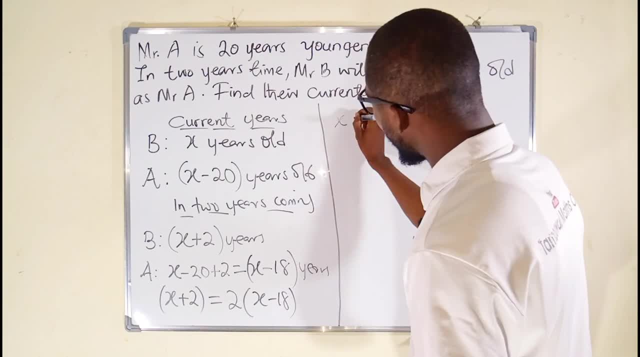 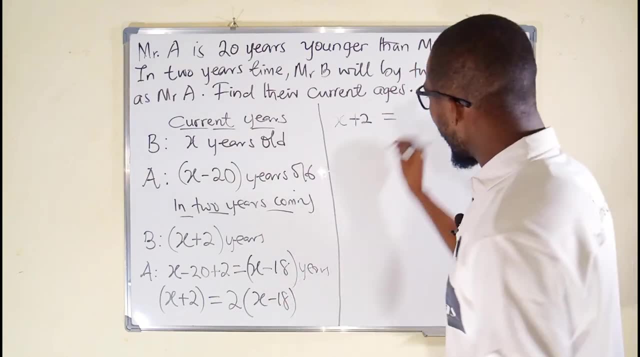 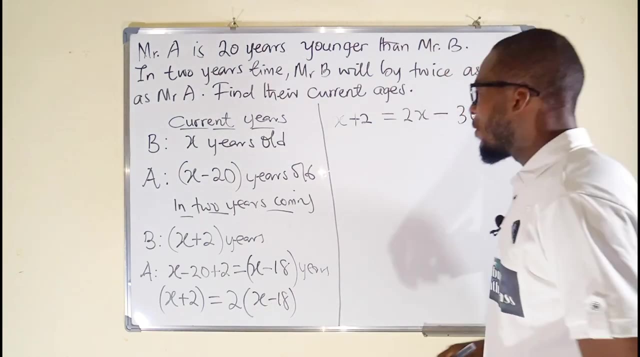 You can see, we have x plus two to the left and to the right. we have two multiplied by x is to x minus two multiplied by 18 is 36.. Let us collect the like terms. You see, we have x here. we have x here, so we bring them. 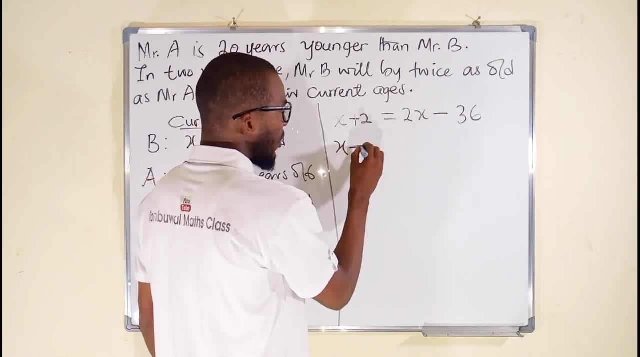 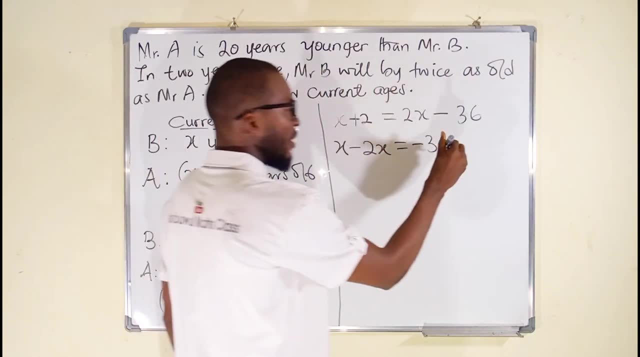 together, we have x. this one is positive. coming to the left, it becomes negative. 2x. and to the right we have minus 36. there, this one is positive. crossing over, it becomes negative as well. so we have minus 2. this is minus x. and to the right, we have minus 38. minus will cancel minus. finally, x. 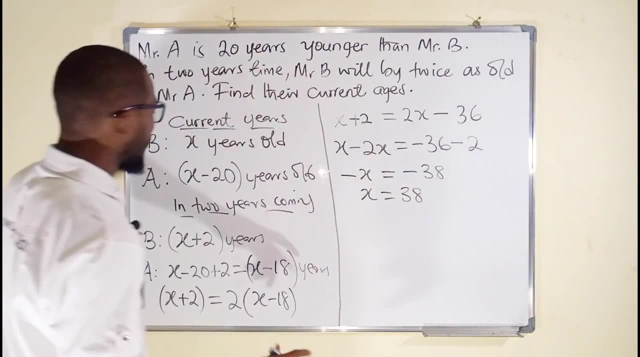 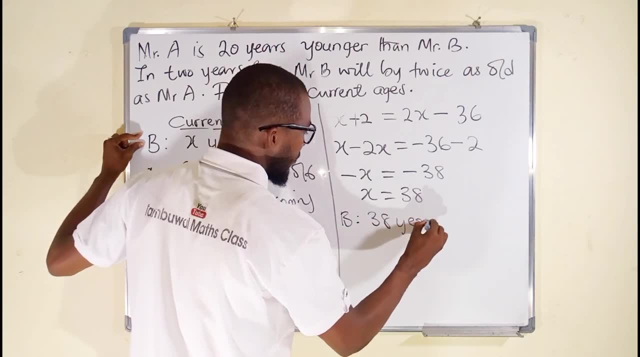 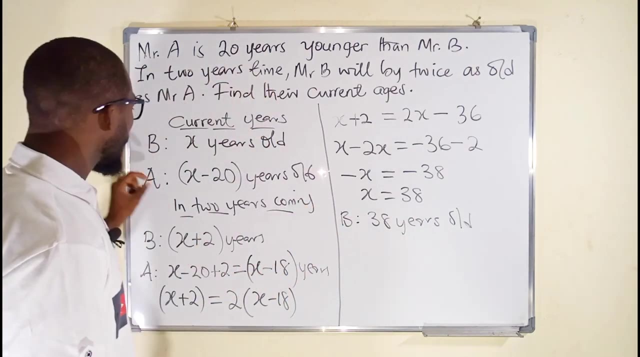 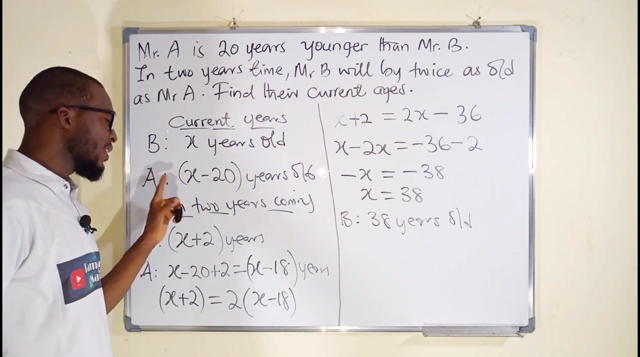 is equal to 38. what does this mean? it means that mr b currently is what? 38 years old. so if mr b is 38 years old, what is the age of mr a? it is going to be 38 minus 20, because we learned that if you subtract 20 from the age of mr b, you're going. 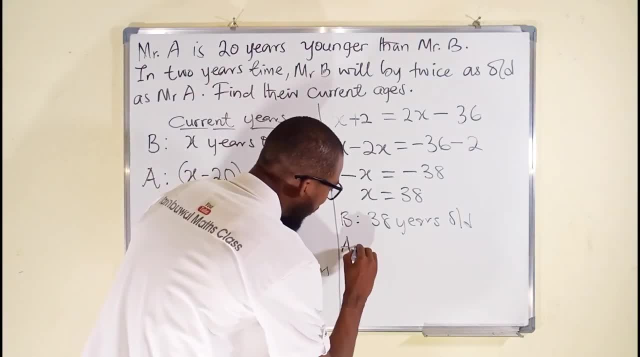 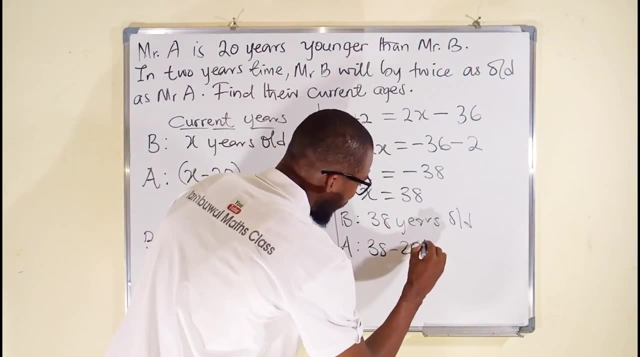 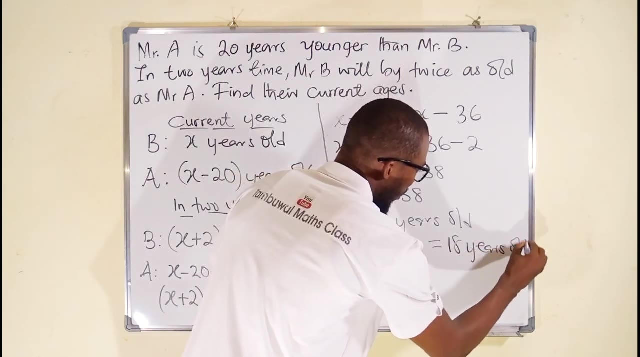 to get the age of mr a. so for mr a it is going to be X minus 20, but X is 38. so we have 38 minus 20, which is equal to 18- yes, 18 years old. so currently mr B is 38 years old, while 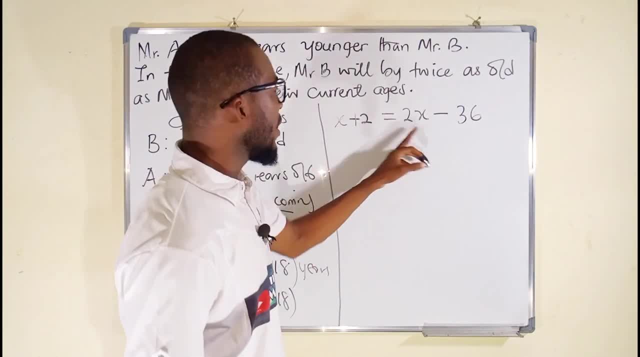 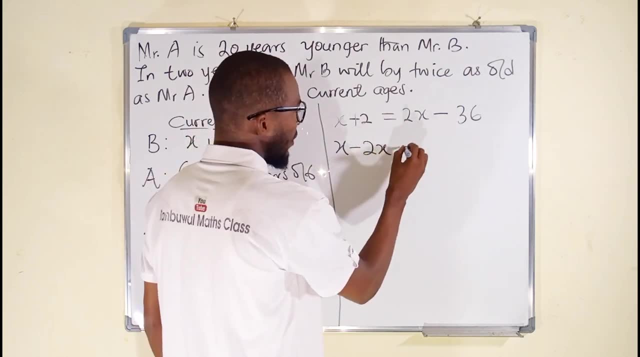 Let us collect the like terms. You see, we have x here, we have x here, So we bring them together. We have x. This one is positive. Coming to the left, it becomes negative 2x. And to the right we have minus 36 there. 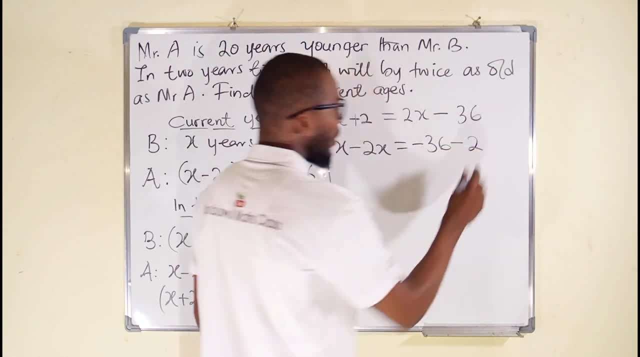 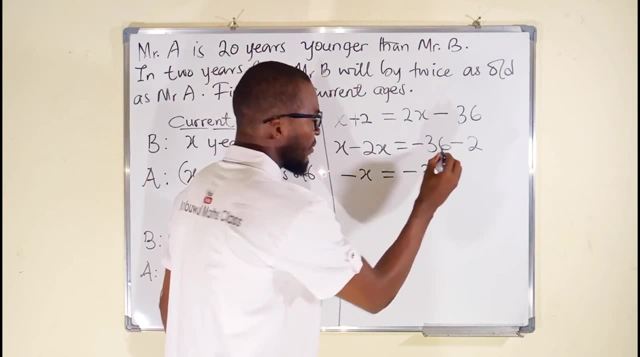 This one is positive. Crossing over it becomes negative as well. So we have minus 2.. This is minus x, And to the right we have minus 38.. Minus will cancel minus. Finally, x is equal to 38.. 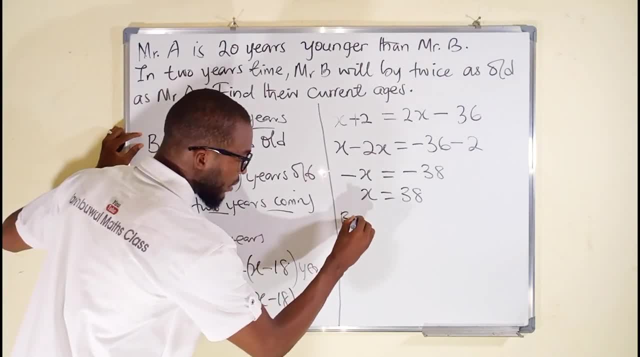 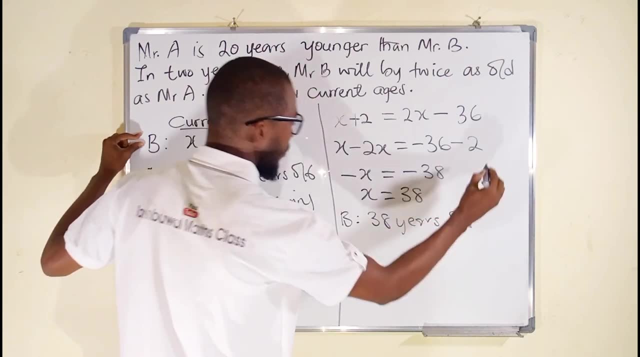 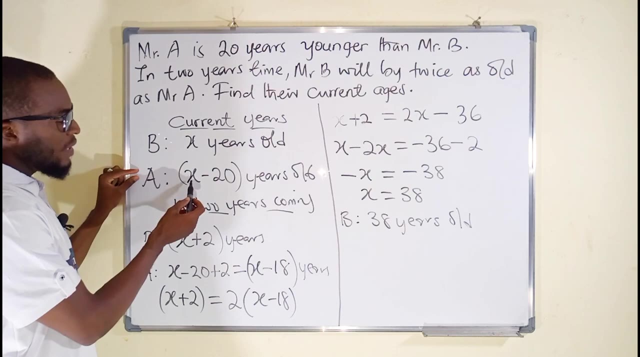 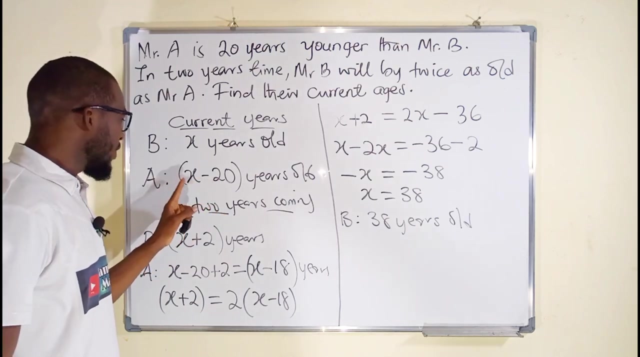 What does this mean? It means that Mr B currently is- what? 38 years old. So if Mr B is 38 years old, what is the age of Mr A? It is going to be 38 minus 20, because we learned that if you subtract 20 from the age of Mr B, 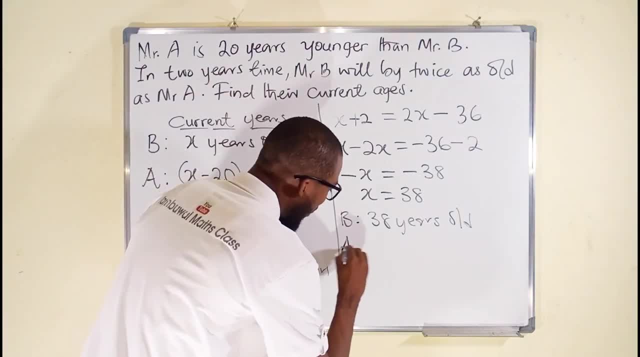 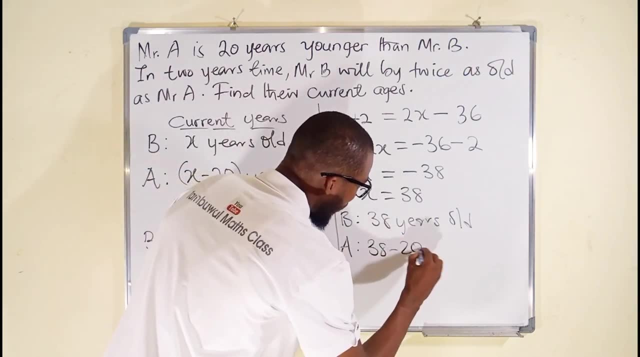 you're going to get the age of Mr A. So for Mr A it is going to be x minus 20, but x is 38. So we have 38 minus 20,, which is equal to 18 years. 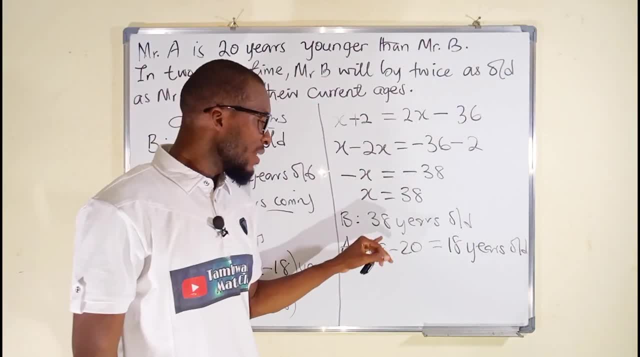 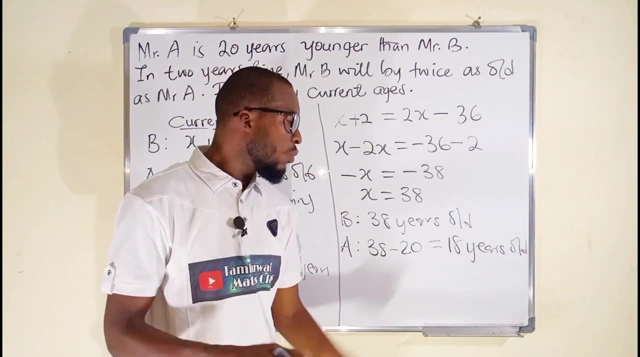 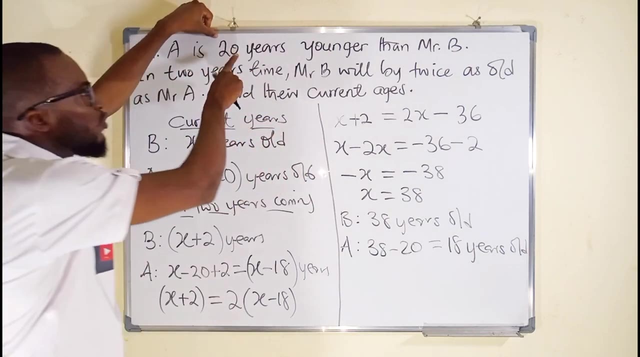 18 years old. So currently Mr B is 38 years old, while Mr A is 18 years old. How can we confirm whether this is true or not? Let us read the statement. The statement says: currently Mr A is 20 years younger than Mr B. 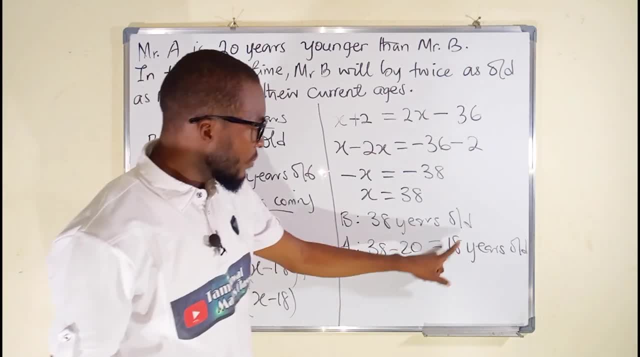 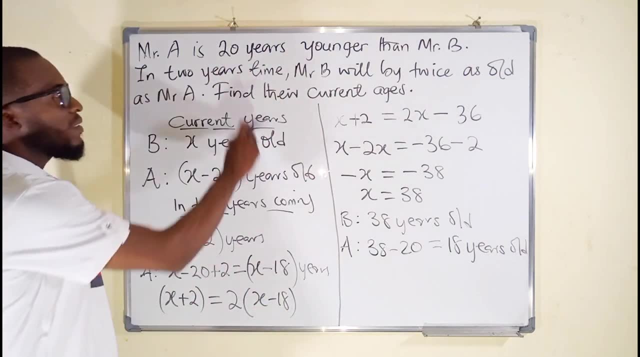 Can you see the difference? The difference between 38 and 18 is 20.. So this statement is true. Let us take the other one. It says: after 2 years, Mr B will be twice as old as Mr A. 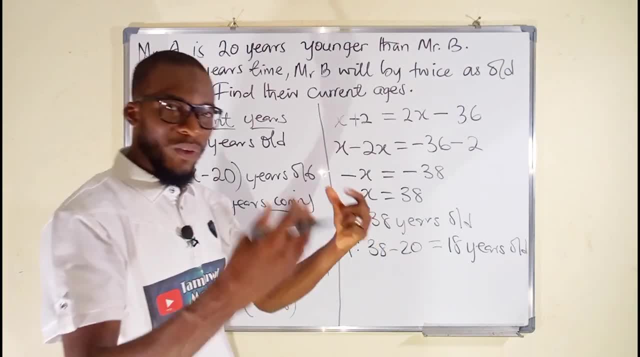 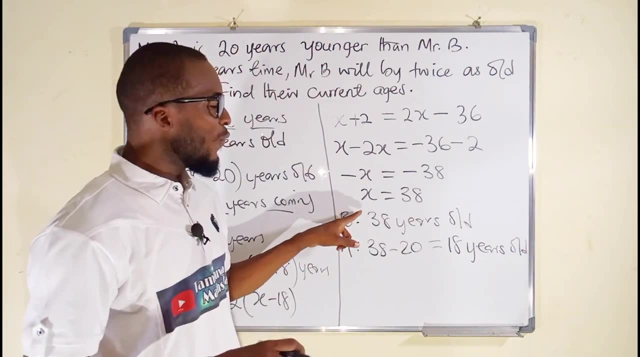 So if we add 2 years to this 38 years, we're going to obtain 40. If you add 2 years to this 18 years, you're going to obtain 20.. You can see that 40 is twice 20.. 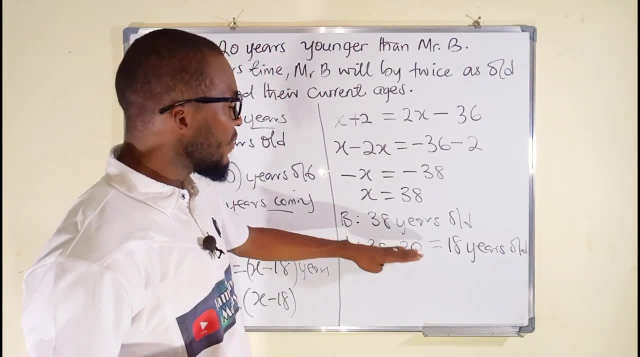 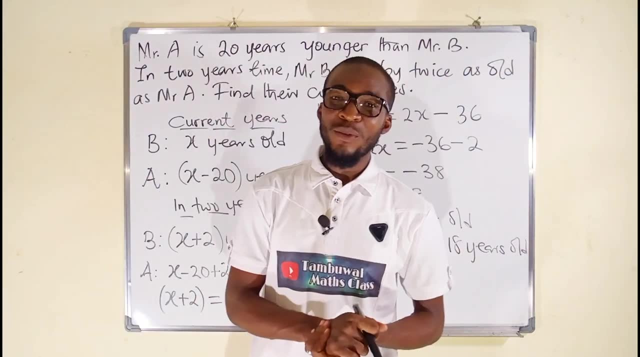 So the answer is correct. Currently, their respective ages are 38 and 18, respectively. Thank you for watching. Do share to your learning colleagues and don't forget to subscribe to my YouTube channel for more exciting videos. Don't forget also to hit the like button. Bye, bye.